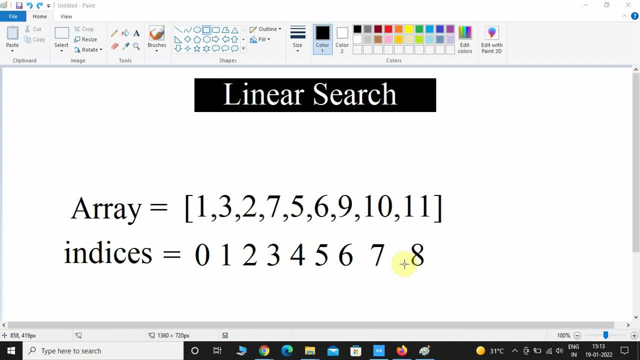 Hey, what's up guys, welcome back. In this video we are going to see how the linear search algorithm works and also we will write linear search algorithm program in javascript. First let us take a look at how linear search algorithm works and then we will write the program for. 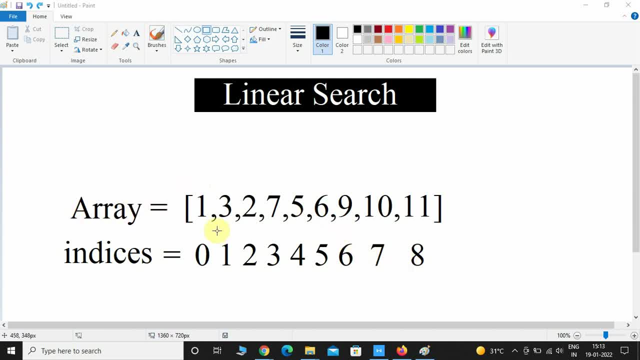 it. So here is an array and it contains few elements in it and these are the indices of those particular numbers. So first let us assume that we want to calculate the index of 2.. So index of this number. So what linear search algorithm will do, is it will linearly? 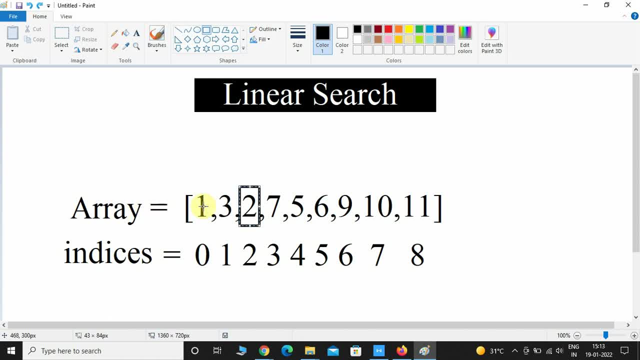 iterate through array, through this array, and then if the key value matches with the particular number, then it will return that index. So here in this example we are trying to find the index of 2.. It will linearly search and if it finds the key 2 then it will return. 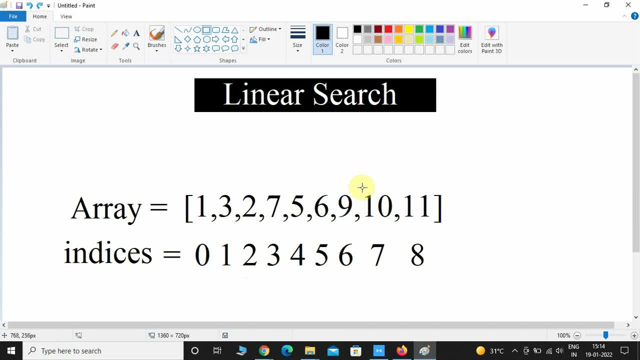 2. Now let us assume that we want to calculate the index of 10.. Again, it will linearly iterate, So it will linearly check all these numbers and then, if it finds that number, it will return the index of that number. What if it doesn't find any? if it doesn't find that key, it will 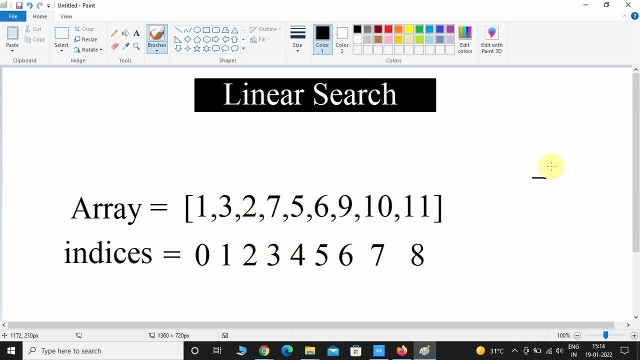 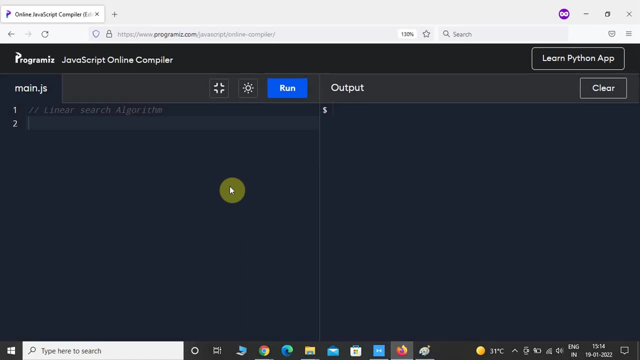 see in this particular array, then it will simply return minus 1.. Now let us see. now let us write a program for this linear search algorithm in javascript. So here I am in the editor, So let me take a full screen. So first things first. what I am going to do is I am 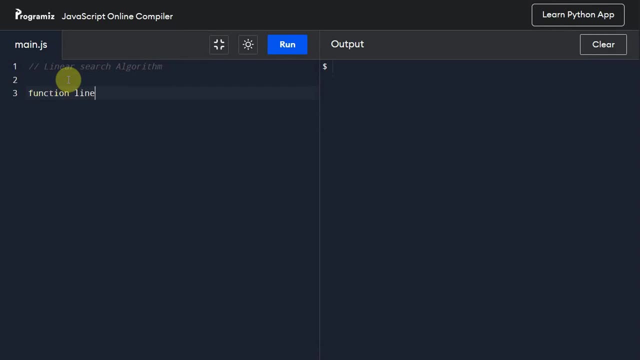 going to define a function called linear search, Linear search. It will accept the function linear search. So it will accept the function linear search. It will accept two parameters. So first parameter is list or array, whatever you want to call it, and also it will accept the key. Okay, So let us leave it empty for now, Before writing. 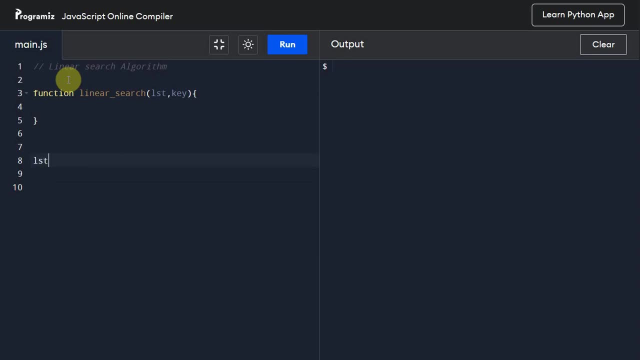 the logic. first let us create a list or array, So it will have few elements: 1, 3, 4, 5, 7, 8. It doesn't have to be in sorted. It may or may not be in sorted order, It doesn't matter. 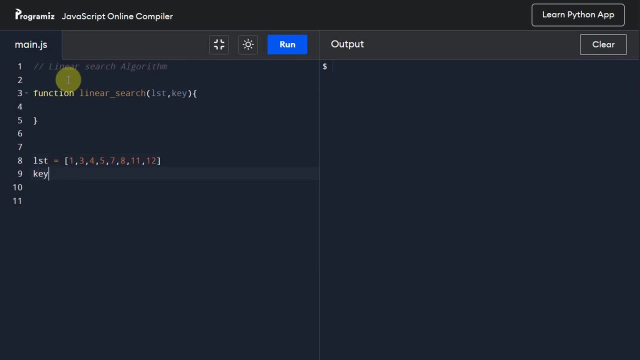 for linear search. Now let us also assume we want to find the index of 4.. So I'll give key value as 4 and I will print this console dot log and we will call this linear search algorithm Linear search and we will pass. 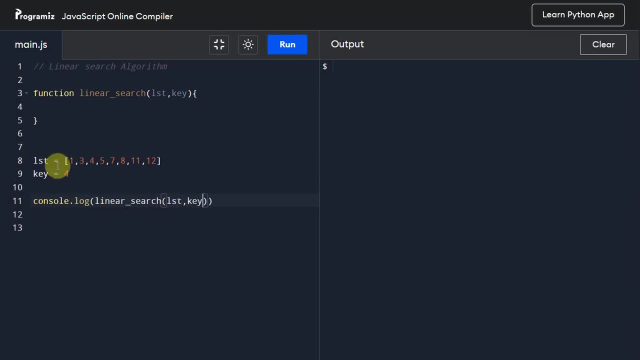 this list and key. So now that we have this driver code ready, let us fill out the logic. For I equals 0.. First we'll take a for loop for iteration: For I equals 0.. I is less than list dot length and we will increment that I value after every. 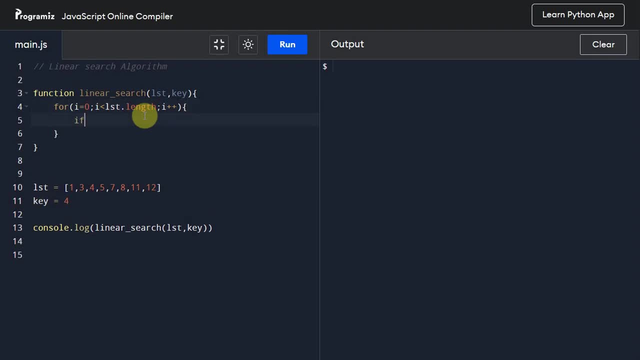 iteration. okay, Now let us take if condition. if list of I matches with our key value, Then we will simply return that I value. okay, So what happening here is it will iterate through this list if. if this key value, that is for if this for list of that in dice index, matches with a key value, then 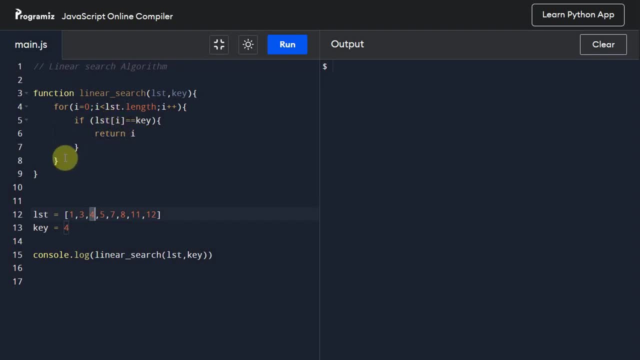 we will simply return that index value. so if it doesn't find any, if it doesn't find key value in this particular list, then it will simply return minus one. so for that we will. we have to give the return outside this for loop. so return minus one, alright. so it is very simple algorithm and the coding part is over. 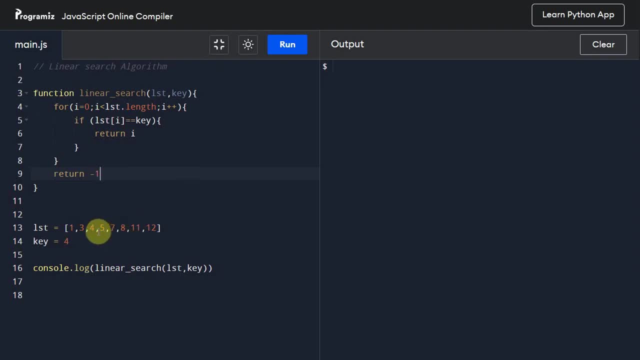 now let us execute this program and let's see whether we get index of 2, because 4 is present at index 2. ok, now let us execute this and here we can see it has printed out 2. now let us check for other values as well. now let me give.